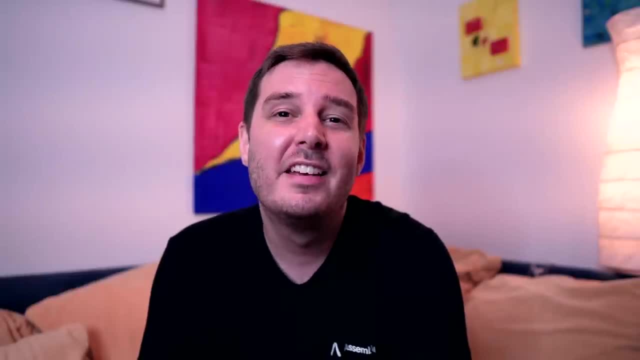 I will mention a few more tips about the job search in the end. so let's jump into the study plan. The first thing I recommend is to lay the foundation with some math basics. Now you might say math is not really necessary anymore, and this is partly true. 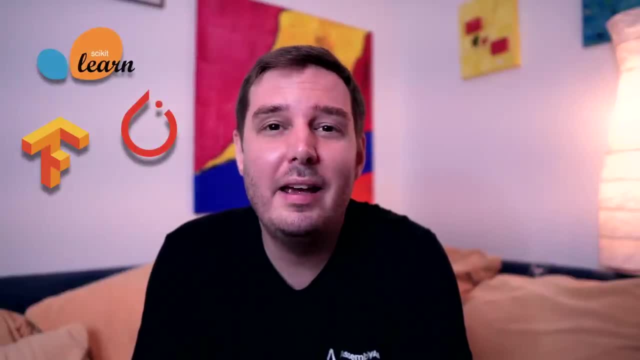 The available machine learning frameworks abstract the math away, and I know many machine learning engineers who don't need it in their day job at all. However, in my opinion, knowing the underlying math provides you with a better foundation and better understanding of how the algorithms work. 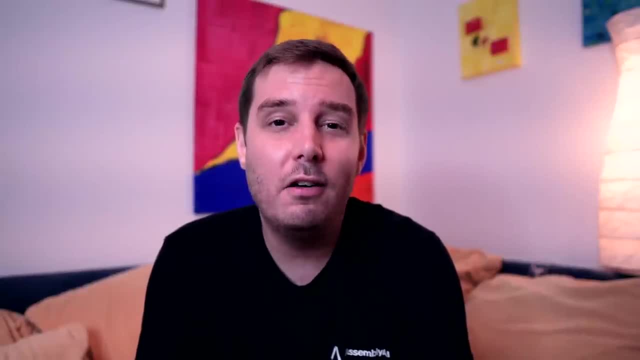 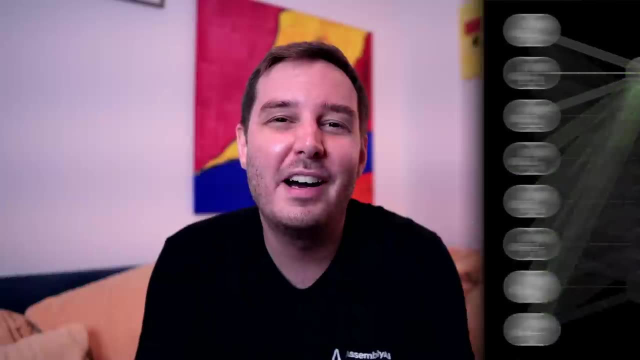 and it makes your life easier when you run into problems. Also, I think there is beauty in the underlying math that makes the machines learn. so, for me, knowing the math sparked my excitement even more. Now you don't need to get too deep into this. 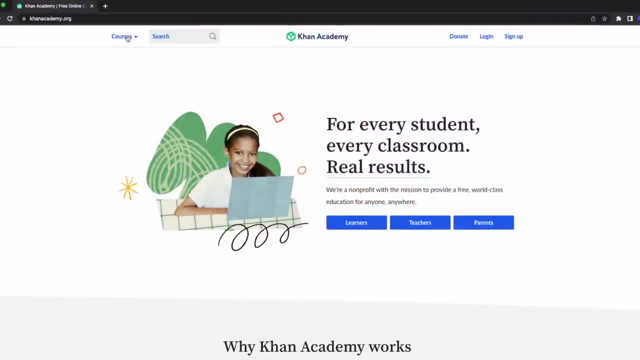 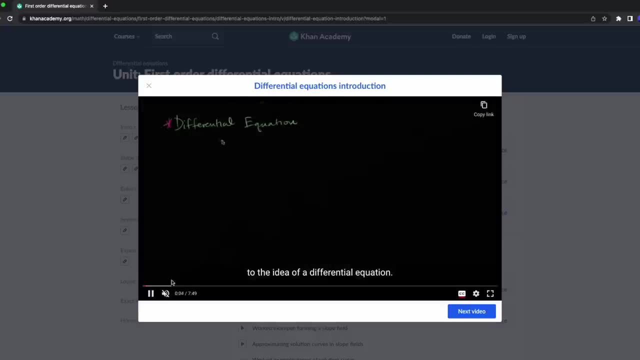 A great website with free resources is Khan Academy. so my recommendation is just to take some basic courses and then move on, and then later, when you do the actual machine learning course and don't understand everything, then come back here and learn the missing topics. 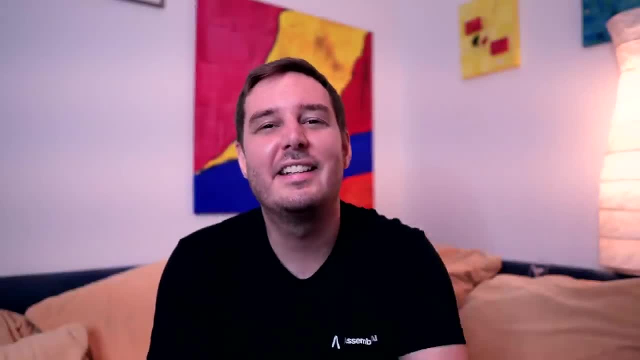 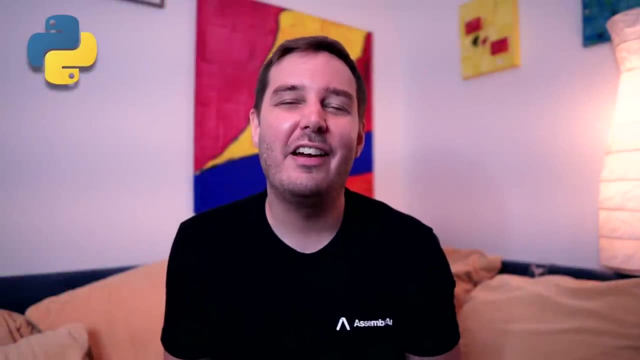 Oh, and, by the way, you find all the resources and recommended courses in the description below. The next step is to learn Python. It is the number one programming language for machine learning and there is no way around it. All major machine learning frameworks are built with it. 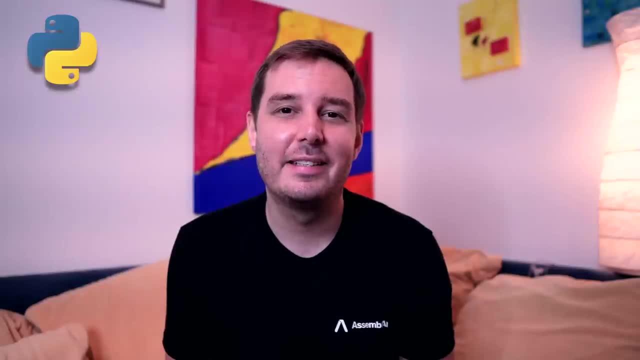 and all major courses use Python for their exercises, so having decent Python skills is essential to build machine learning projects. Now you don't need to become an advanced software developer, but a little bit more than the beginner level would be great. One great thing about Python is that it is very beginner-friendly. 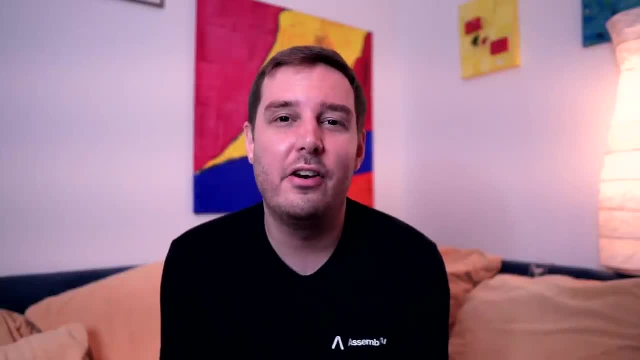 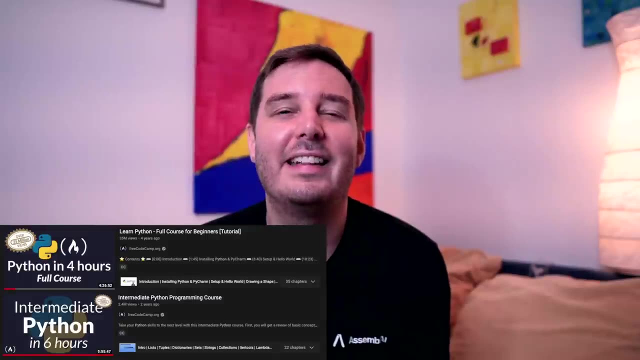 and in my opinion it's the best first programming language you can learn. I recommend two free courses- one 4-hour beginner course and one 6-hour intermediate course- and then you should have a solid base. This step is what I call the machine learning tech stack. 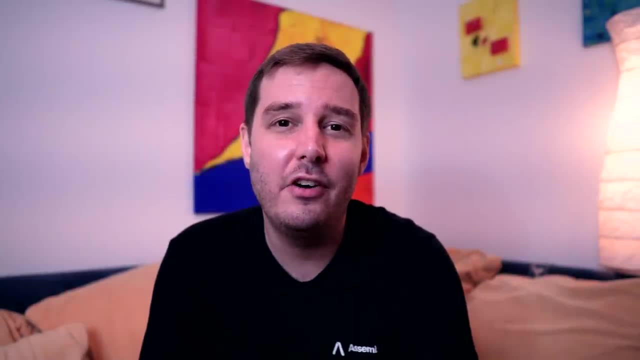 and consists of the most important Python libraries for machine learning, data science and data visualization. This step is a bit optional because you can also pick up these skills later when you do the actual machine learning course, but I think it's great to build the foundation first. 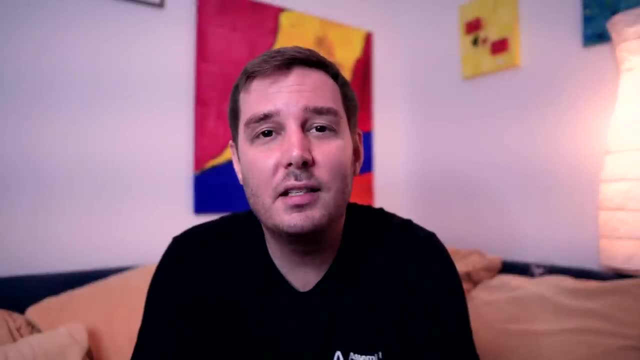 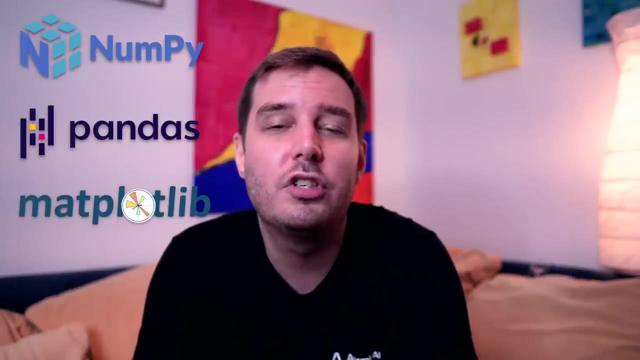 and then it will be easier later. The three libraries I recommend at this point are NumPy, which is the base for everything, Pandas, which is important for data handling, and Matplotlib, which is needed for visualization. These libraries are used in almost every machine learning project. 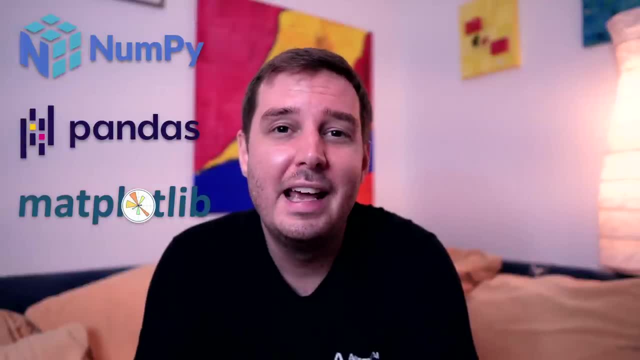 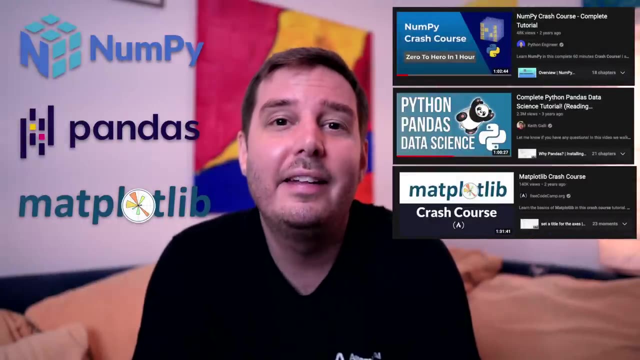 that's why I would include them in your learning path at this point. Again, you don't need to learn too much here. I recommend just following one free crash course for each library and then later pick up more advanced concepts if you need them. 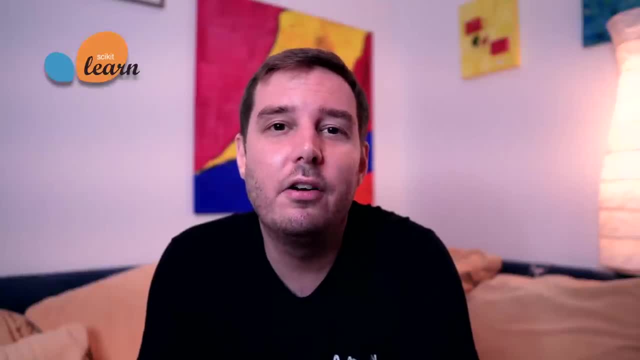 At this point. you don't have to learn the machine learning courses like scikit-learn, tensorflow or pytorch. You could, of course, if you want, but these are included in the machine learning course. I show you in a moment so you can pick these up later. 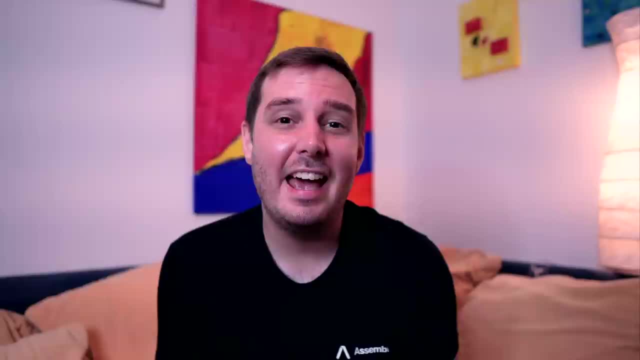 Now that we've covered the coding skills, it is finally time for the actual machine learning course. There are many great ones available, but the most popular- and in my opinion, also one of the best ones- is the machine learning specialization by Andrew Ng on Coursera. 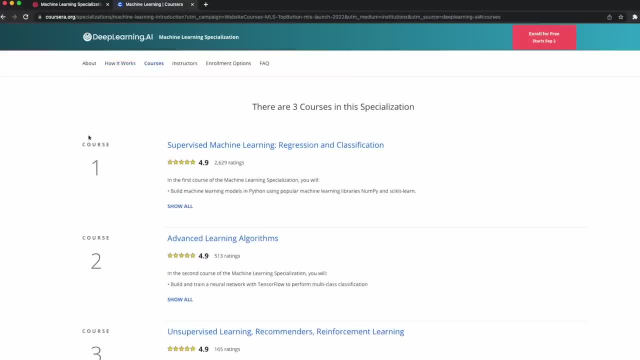 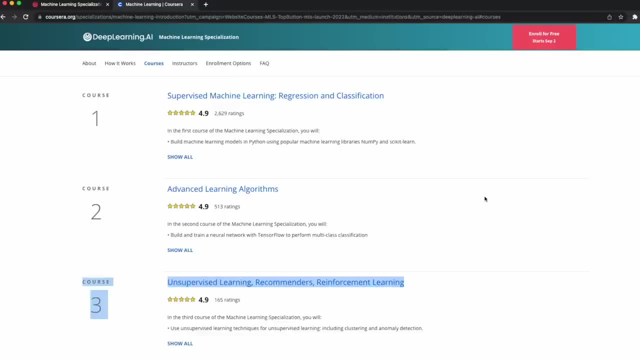 This specialization includes three courses. it got revamped just a few months ago and now includes Python with NumPy, scikit-learn and tensorflow for the code, You not only learn all the essential machine learning concepts, but also get your first hands-on experience with the ML libraries. 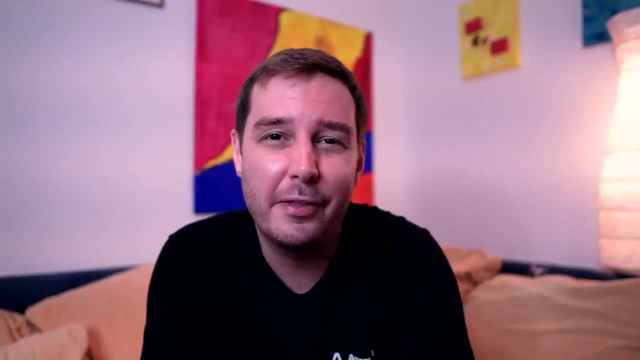 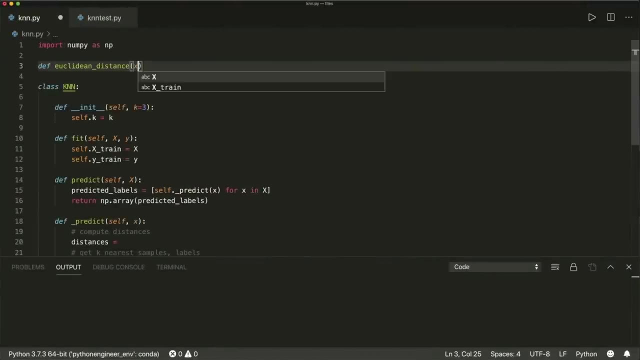 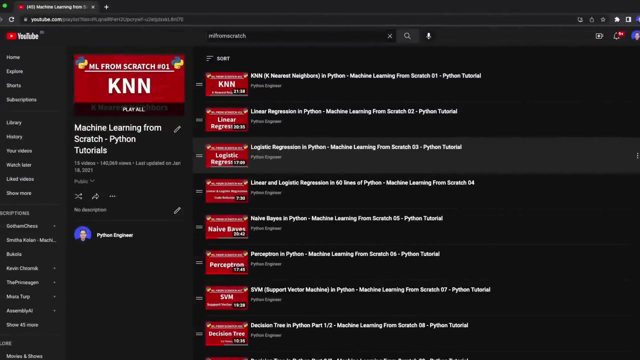 It is extensive and it takes several weeks to finish, but it's worth it. After these courses, I have one more recommendation for you. I suggest to implement a few algorithms from scratch in Python using only pure Python and NumPy, For example, by following my ML from scratch playlist here on YouTube. 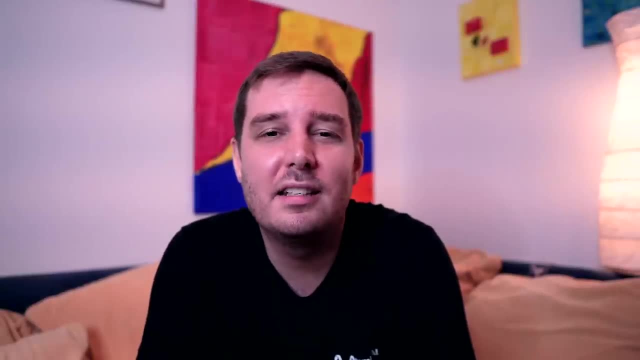 This is completely optional, but it helped me to properly understand some of the concepts from Android, and a lot of students have told me the same feedback, so check it out if you want to. Also, we plan to release an updated version of the ML from scratch course. 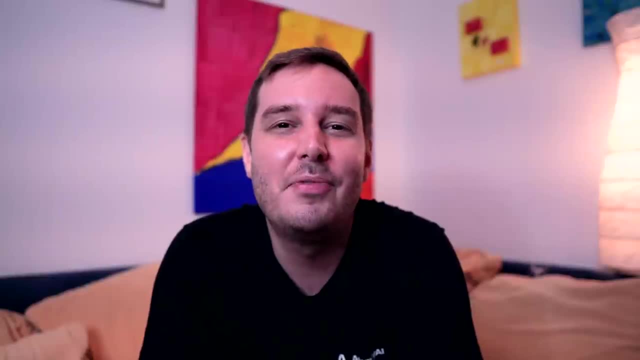 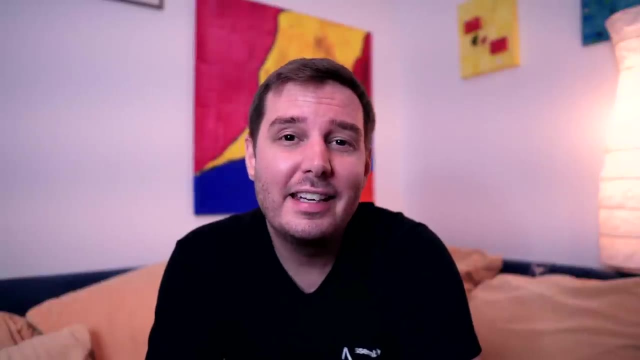 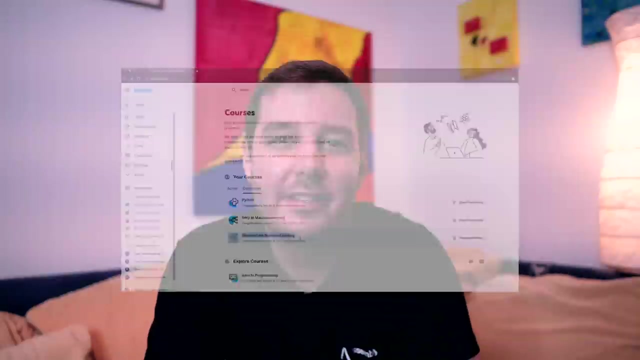 here on the Assembly AI channel, so make sure to subscribe to our channel and don't miss it. Now. I recommend getting even more hands-on and learning more about data preparation, For this Kaggle has awesome free courses on their website. I recommend at least the Intro to ML and Intermediate ML courses. 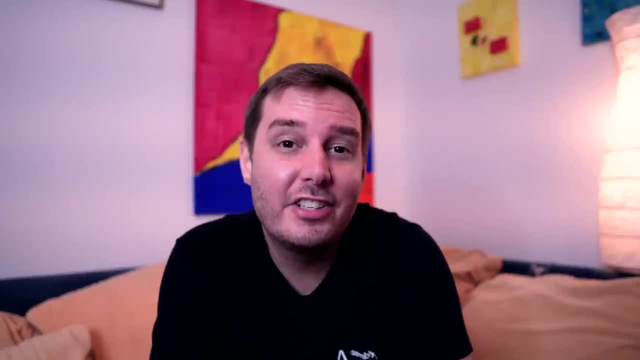 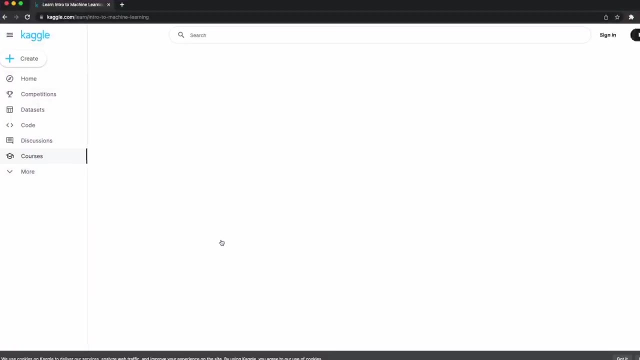 They are lightweight compared to the previous one and some material is just a little bit more complex, but you'll learn more about data preprocessing and data preparation with pandas. Each lesson has a theory part and then some coding exercises. It also gives you a gentle introduction to the Kaggle platform. 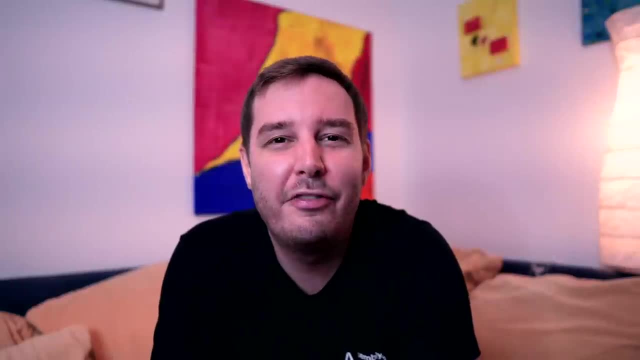 and you learn how to make code submissions on Kaggle, which is perfect for the next point. Now it's time to practice as much as possible and apply your knowledge to real-world machine learning problems. For this, the best platform is Kagglecom. 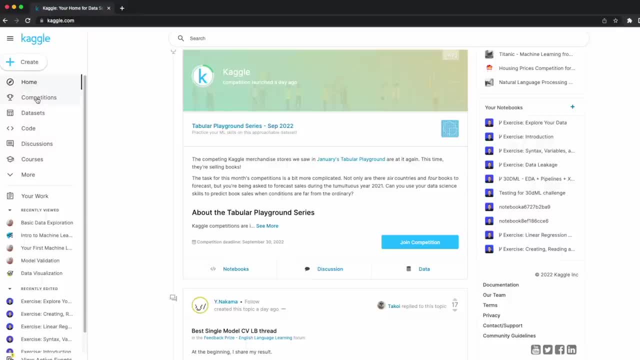 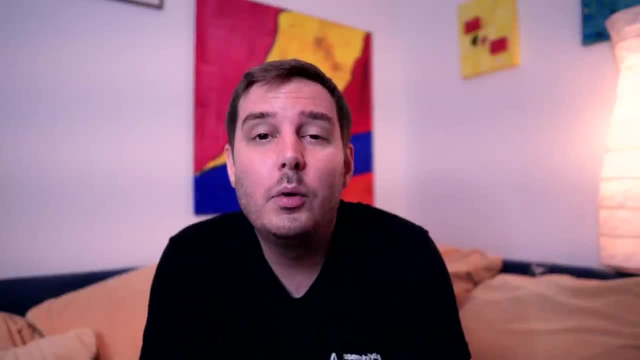 It provides thousands of different datasets and challenges where you can participate. Participating in challenges can motivate you a lot. Now I wouldn't try making it to the top or even winning price money with this, because, to be honest, this requires true expertise and also a lot of GPU power. 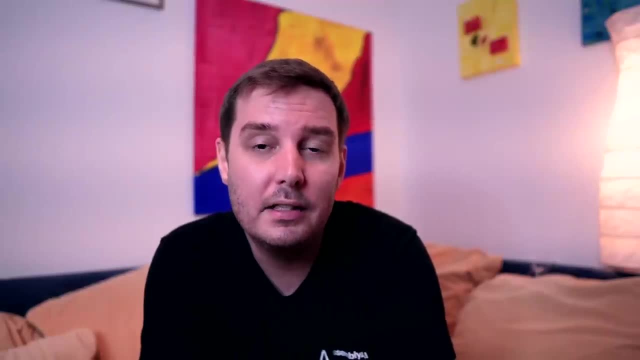 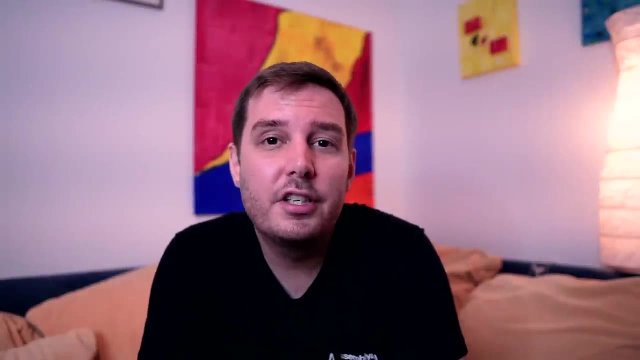 But I would still try to tweak your solutions multiple times by learning more about data preprocessing and also about hyperparameter tuning. You can then use Kaggle competitions to build your portfolio and put them on your CV. So, in my opinion, Kaggle is an awesome platform. 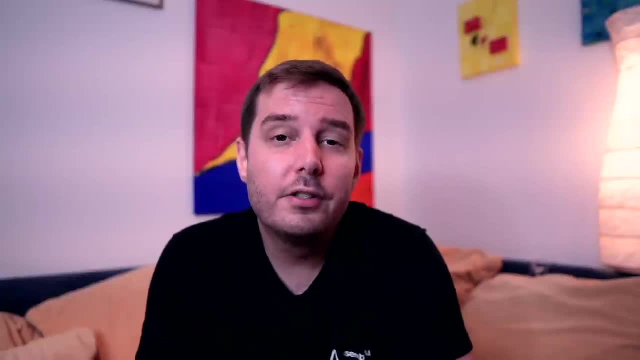 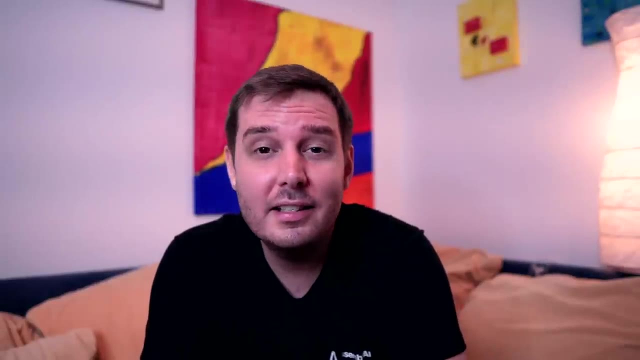 and you should practice here as much as possible. Of course, you can also tackle other machine learning problems outside of Kaggle. It just makes your life a little bit easier because it provides you with the datasets, a platform to evaluate the projects and there's a whole community around it. 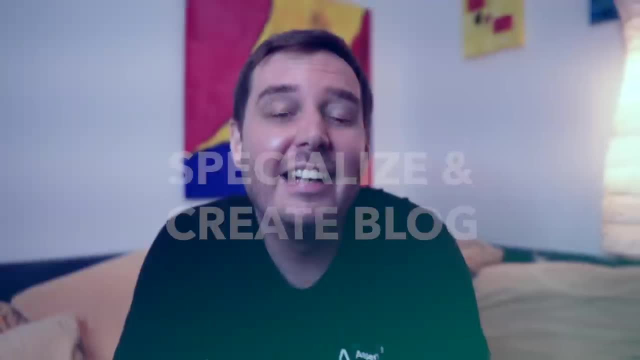 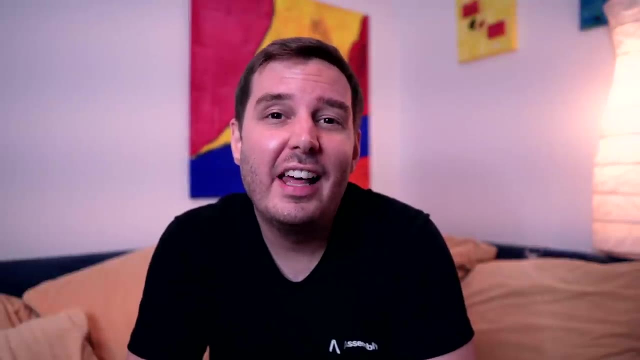 At this point, you can already be super proud of yourself. And now, in this last section, I want to give you a few more tips if your goal is to get a job. The tasks of ML engineers vary a lot, and it's not possible to know everything. 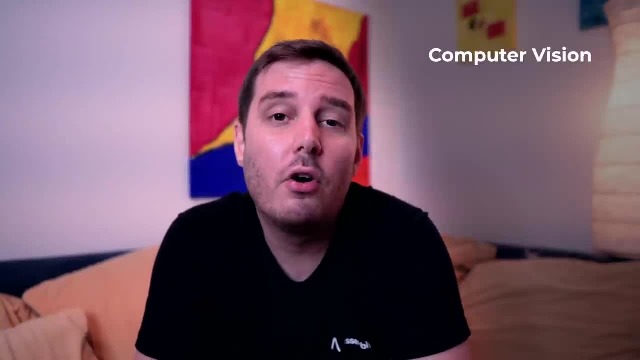 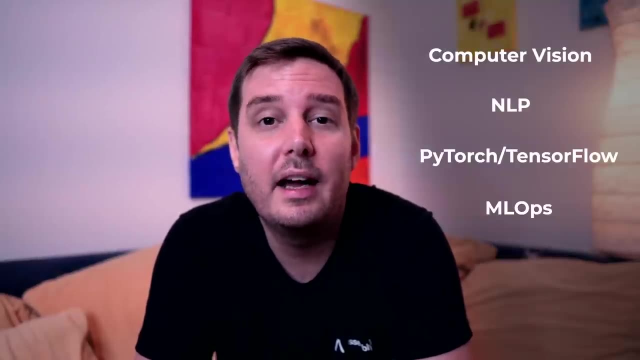 For example, some positions are specialized in computer vision or NLP, or they require you to have experience with a specific ML framework or even MLOps requirements like how to deploy and scale ML apps. MLOps is a whole field on its own. 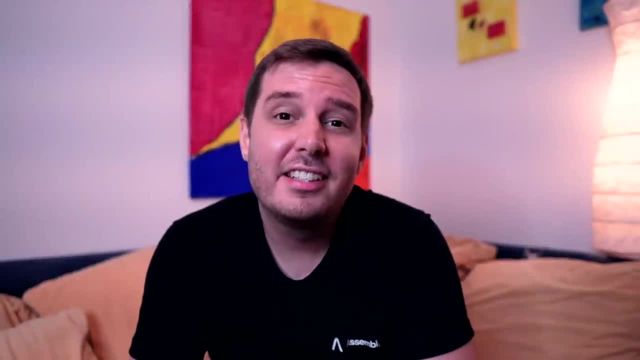 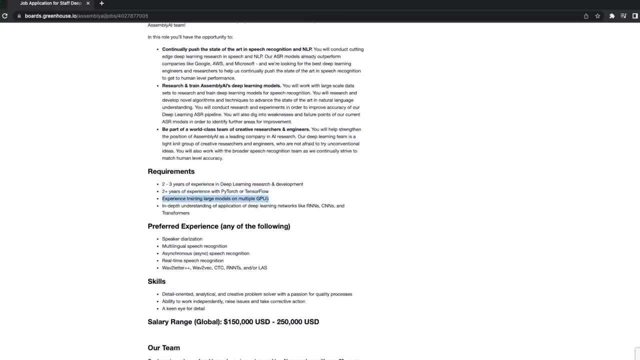 so I may cover this in a separate video. My point is: you have to decide in which field you want to work and then look at the requirements in some corresponding job descriptions and then specialize in this direction. Another great tip I can give you: 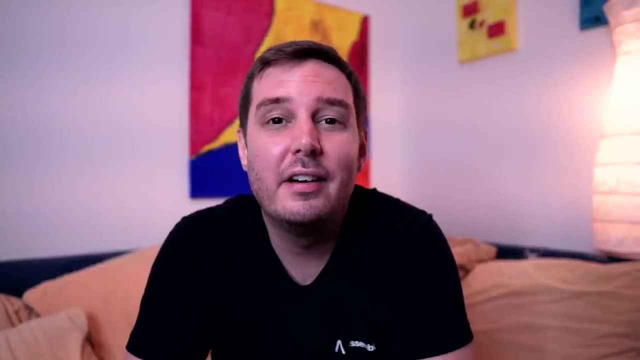 and this is something I wish I had done earlier in my career- is to start a blog. You can write tutorials, share what you've learned, which projects you have built, which problems you have faced along the way and how you've solved them.